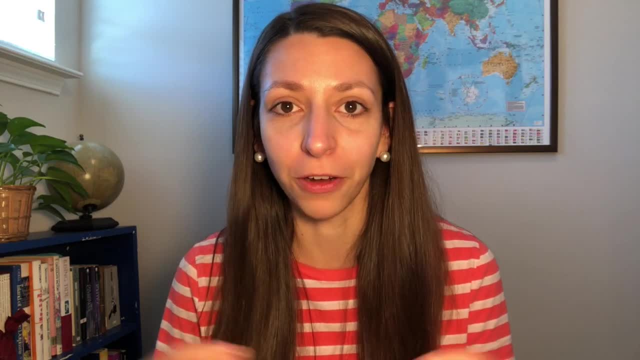 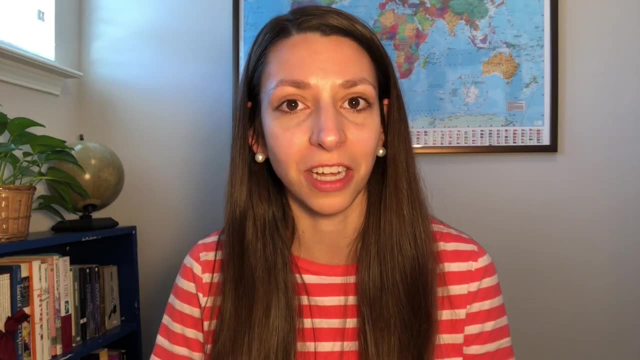 because I do these and there are good hints as to how to figure out my tests, but I know that they apply to lots of other teachers and tests as well, And statisticians have shown this by doing lots of studies on multiple choice tests like the ACTs, the SATs, over years. This is not a video about 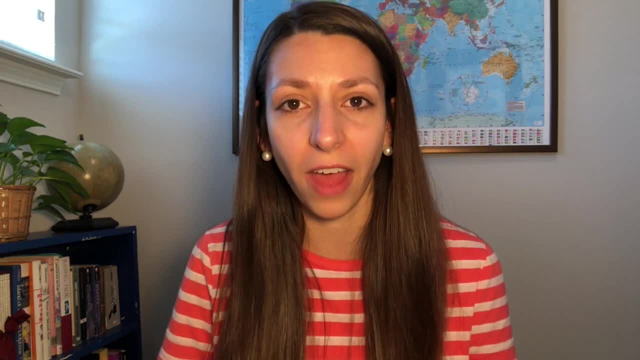 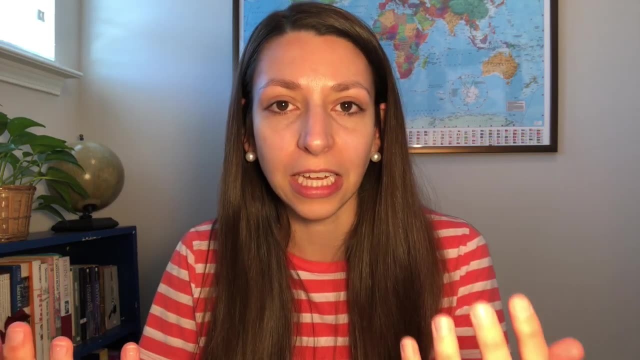 test taking strategies per se. I have a whole other video on that, about how to strategize making educated guesses and doing your best on multiple choice tests with a balance of content and test taking skills. This video is for when you get to that point in your test taking and you come across. 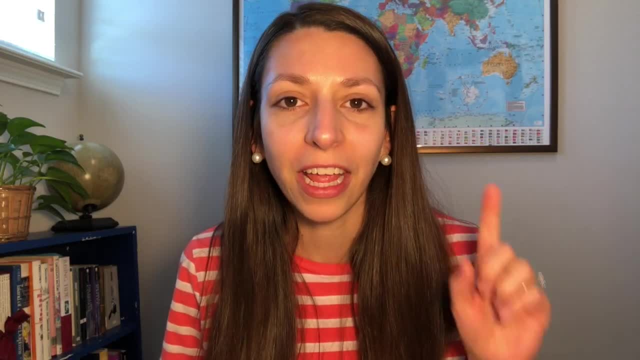 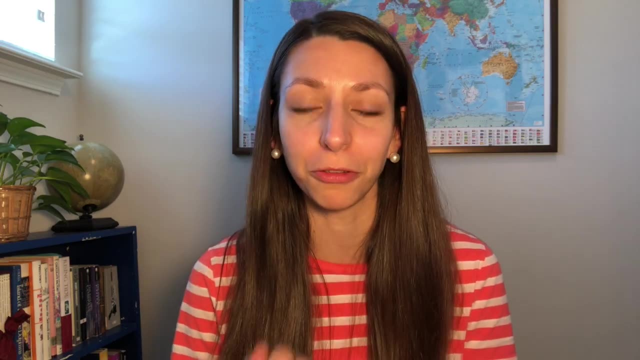 a question you have absolutely no idea, but I'm going to show you how to answer correctly on a multiple choice test without knowing the answer. Again, I'm a teacher. Obviously, I would love for you to learn the content because you want to know it, not necessarily because you. 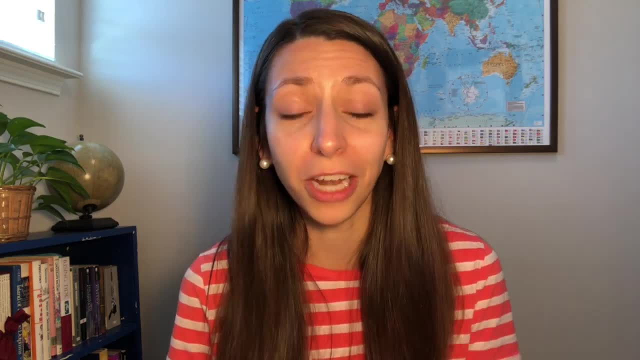 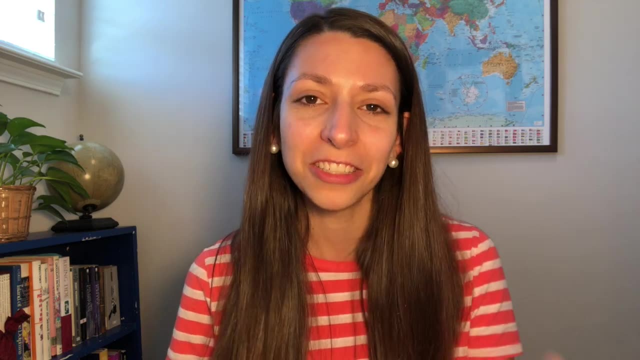 want to get the best grade on the test, but I do know that tests stress a lot of students out, So hopefully you'll find this video helpful for those moments when you get to a multiple choice test and you are totally stuck. So stay tuned for some of my favorite strategies and make sure you let me. 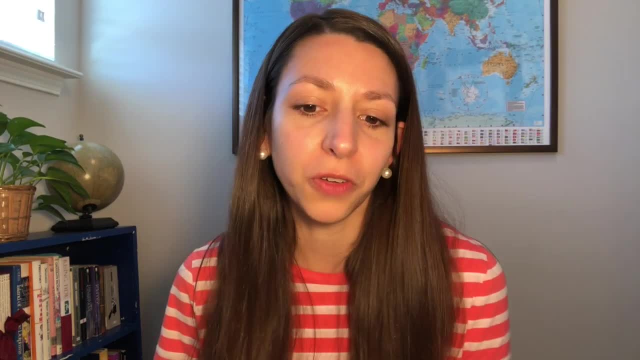 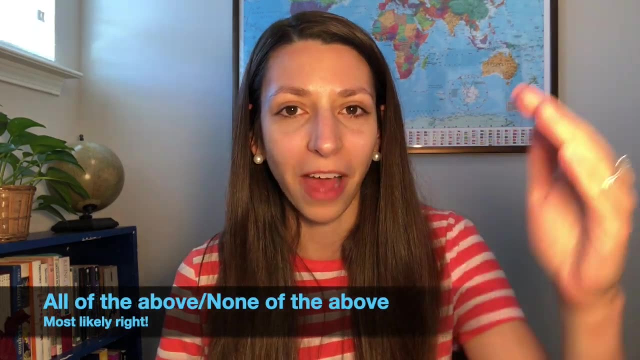 know in the comments if any of these have worked for you. First, multiple choice hack: is that very commonly- and not just for my classes, but all multiple choice tests- it is more likely if you have a list of questions that you want to answer, you can do that by clicking on the link in the 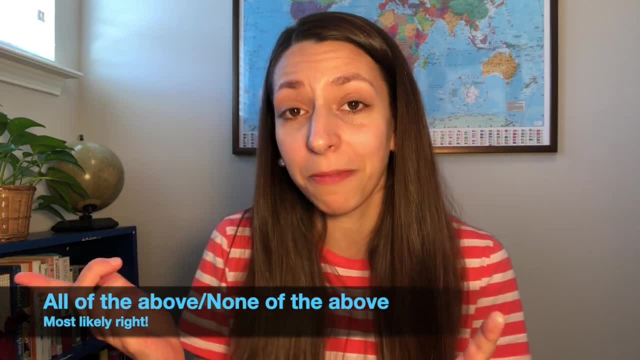 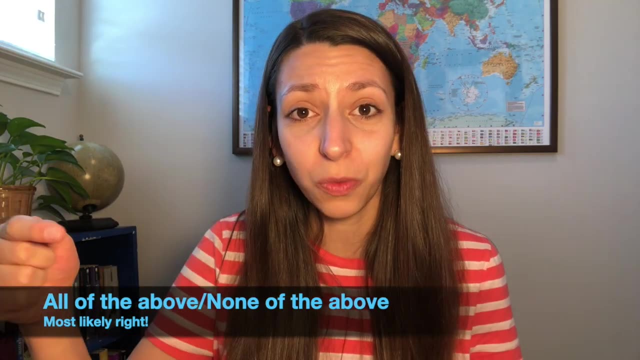 description. If you have a list of answer choices and one of them is all of the above or none of the above, that that is the right answer. Again, statisticians have analyzed lots and lots of different tests and figured out that this one is more commonly right than wrong. So if you see an 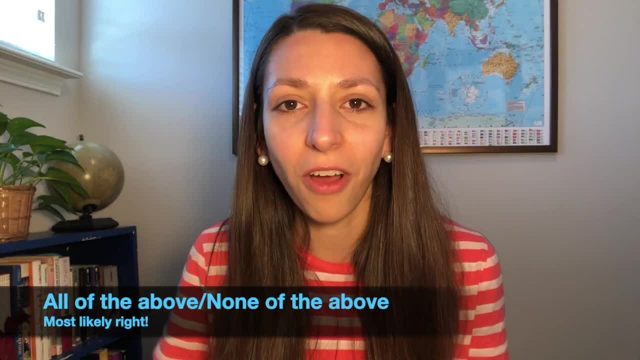 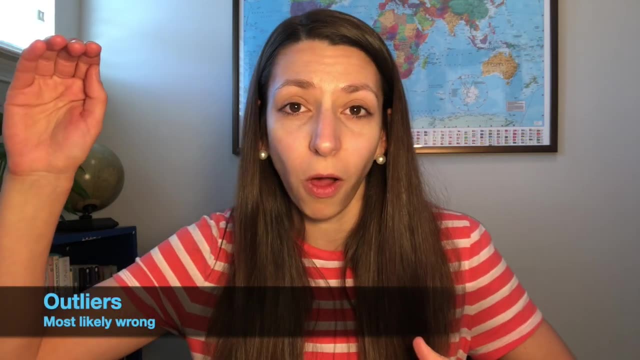 answer choice and you have no idea what the question is asking, go with all of the above. Next up is something to avoid If you see outliers, meaning numbers that are really really big, really really small, or just have nothing to do with the rest of the group of answer choices. 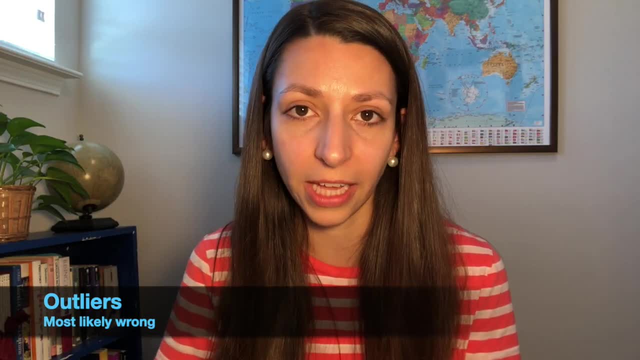 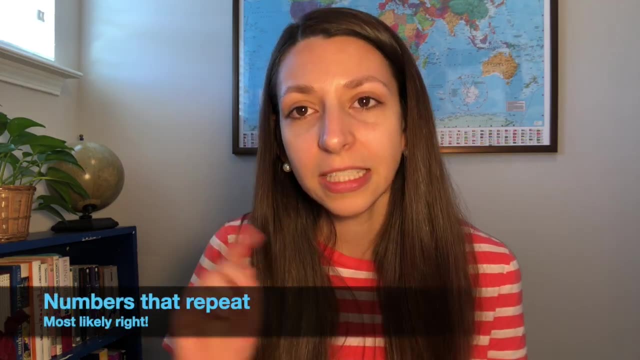 those are probably answer choices to avoid When you are totally guessing. So stick to the numbers that are closer together. If you have a list of numbers as your multiple choice answer choices, The next hack is to look at repeat numbers. This is something I do on my test sometimes. Now, if you have a list of answer, 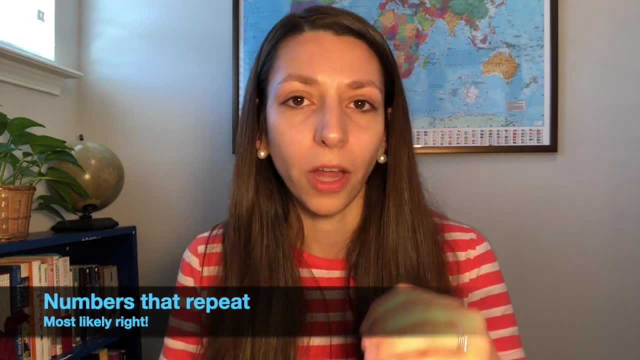 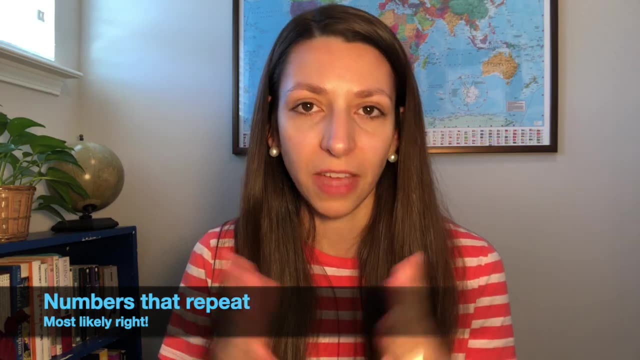 choices that are numbers, numbers that are either close together or numbers that are very similar, could be an indicator that one of those numbers is the correct answer. So sometimes teachers, if they have a math problem, will actually work out the math problem and introduce mistakes. 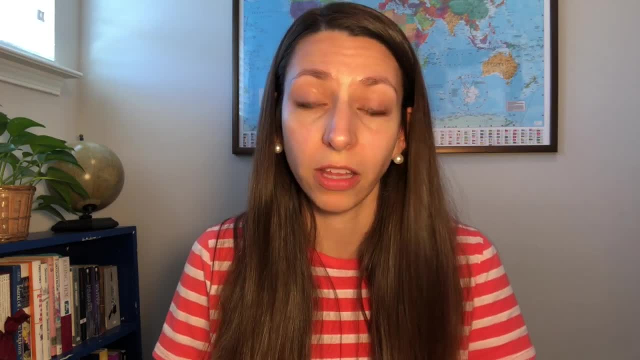 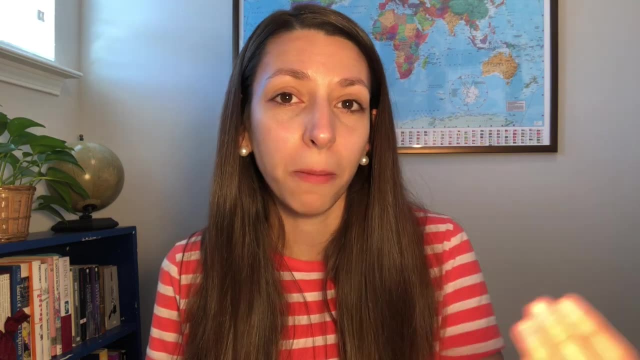 as they're working it out, as if they knew what the students would do incorrectly on the exam and then make those one of the incorrect multiple choice answers. But sometimes teachers can get lazy and they'll just put a number close to the actual answer as an incorrect answer choice. I 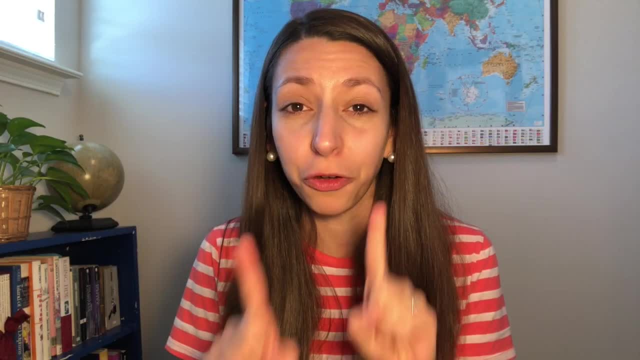 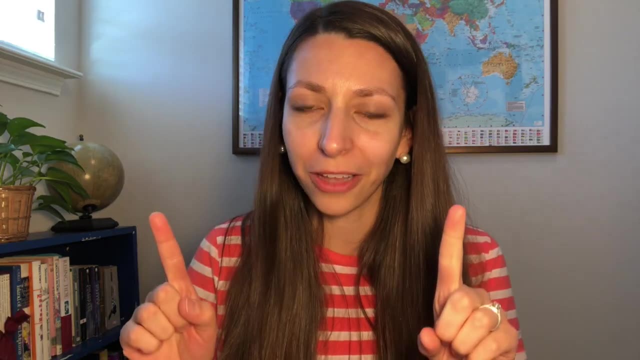 confess I do do this sometimes. So if you see two answer choices that are numerically pretty close together, it might give you a hint that one of them is the correct answer. And remember if you can eliminate at least two answer choices if there are four options on a multiple choice question. 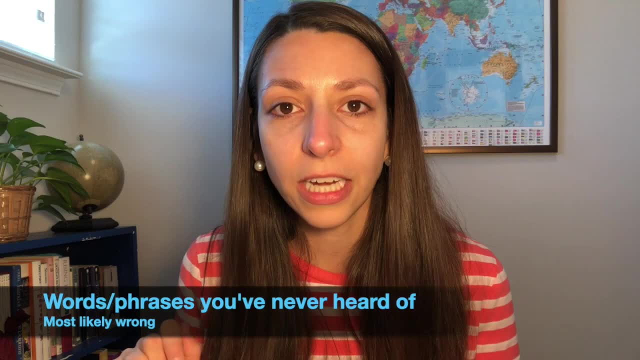 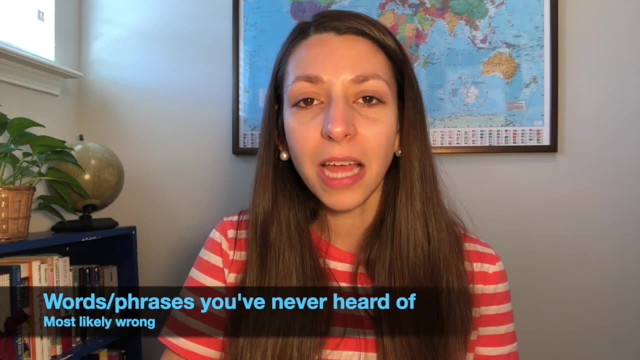 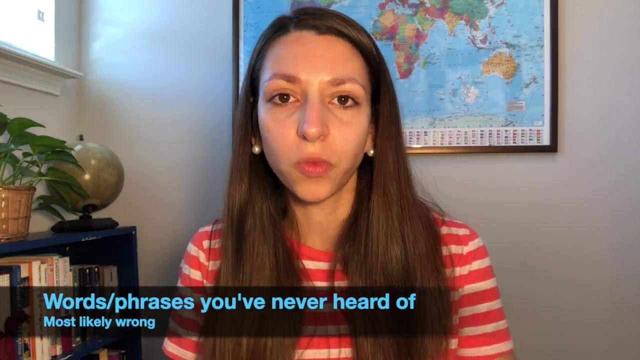 you have a 50- 50 shot Test taking hack number three: I tell my students this all the time, but teachers like to put distractor answers in their multiple choice tests And sometimes these are answers or words or things you've never heard of before. So avoid those answer choices- Any answer choices with words. 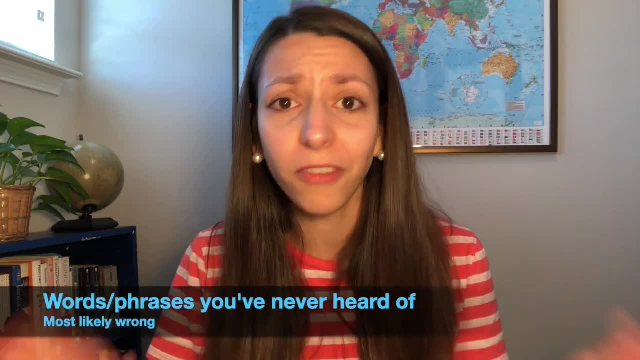 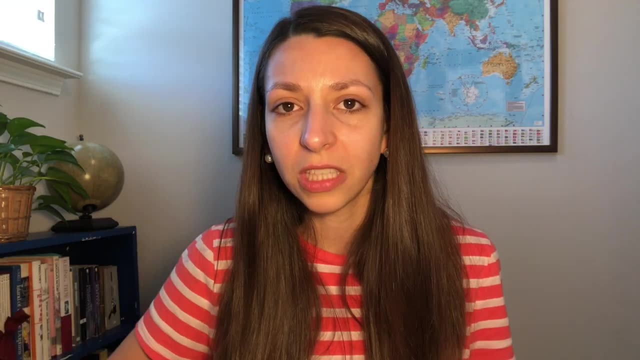 vocabulary, a concept you've never heard of or not covered in your unit in class. don't choose that answer. It's a way to distract from the correct answer So you can avoid those things you've never heard of. My next test taking. 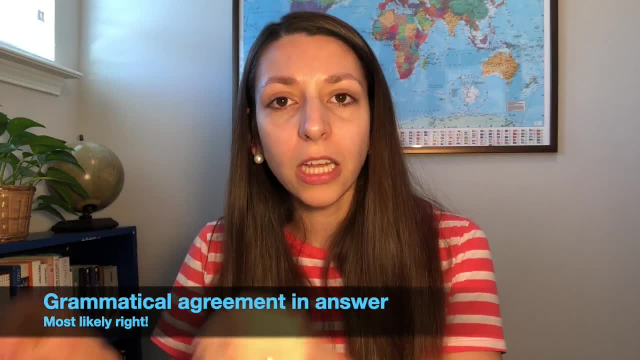 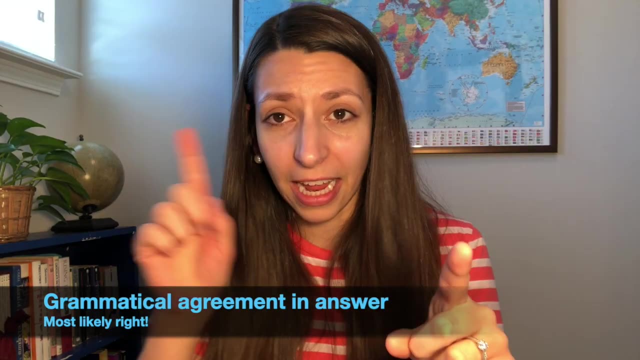 hack is to pay attention to the grammatical phrasing of the question and the answer choices. The one that is correct is more likely to be a matching answer choice. So make sure A's and ands agree with your answer choices. Make sure there's agreement with plural and singular phrases. 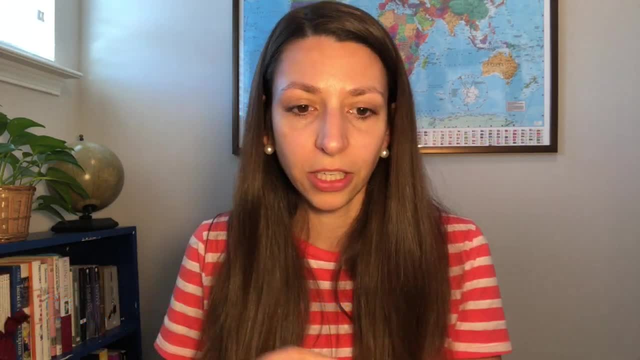 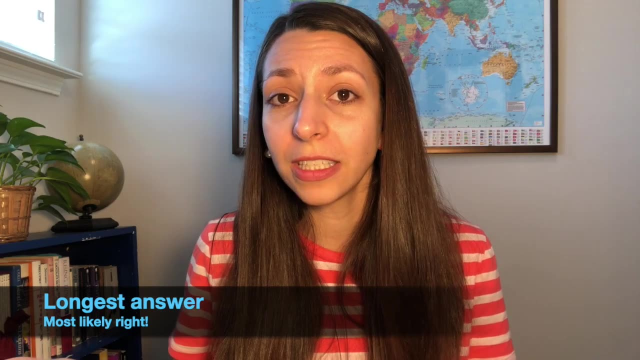 All of these things can actually give you a hint towards the correct answer. Another thing that might give you a hint that the answer is correct is that if it's long or longer than the other answer choices, it's the correct one. Teachers are more likely to spend more time on the correct. 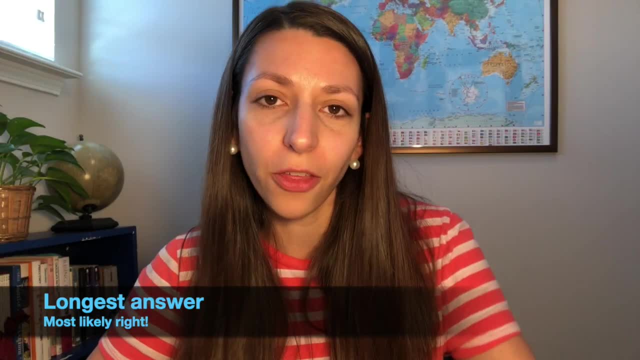 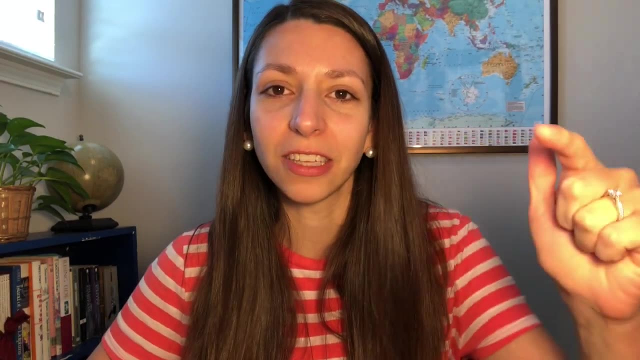 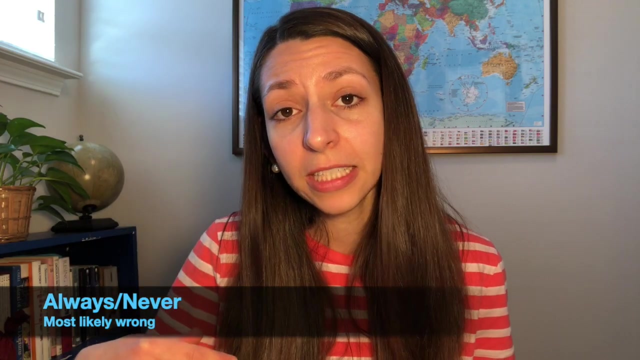 answer, So the right answer might be the longest. This is not always the case, but you could be guessing right if you guessed the longest answer and you have no idea what the actual answer choice is. Another thing to eliminate when you're going through your multiple choice test is phrases. 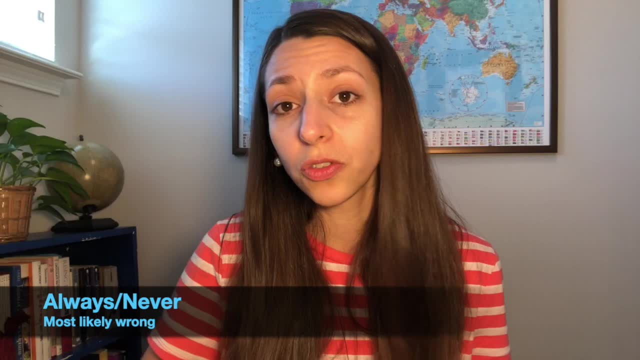 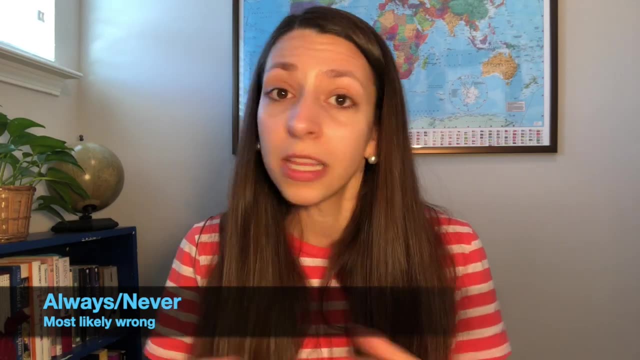 like always and never in the answer choices. If an answer choice has always or never, these are absolutes and most likely are not going to be your correct answer choice. This is not always, but you can make sure. if you're totally guessing, just go ahead and eliminate the always and never.